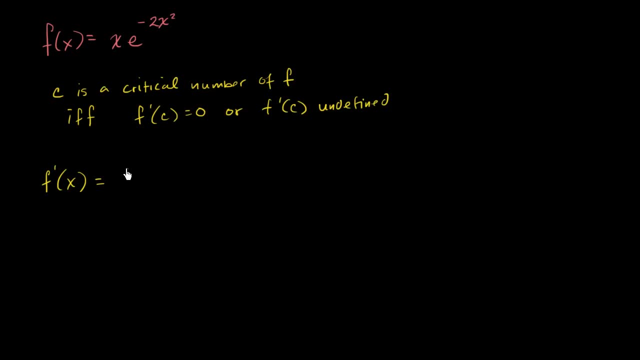 So it's going to be the derivative with respect to x of x. So it's going to be that times e to the negative, 2x squared, plus the derivative with respect to x of e to the negative 2x squared times x. So this is just the product rule. 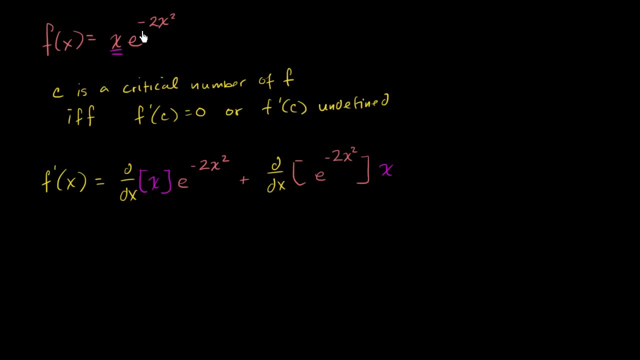 Right over here. derivative of the x times e to the negative 2x squared, plus the derivative of e to the negative 2x squared times x right over here. So what is this going to be? Well, all of this stuff in magenta. 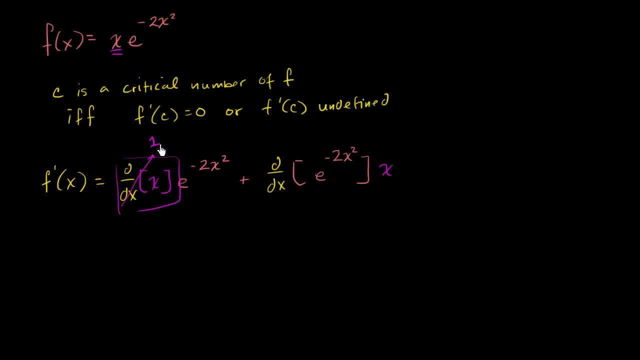 the derivative of x with respect to x, that's just going to be equal to 1.. So this first part is going to be equal to e to the negative 2x squared, And now the derivative of e to the negative 2x squared. 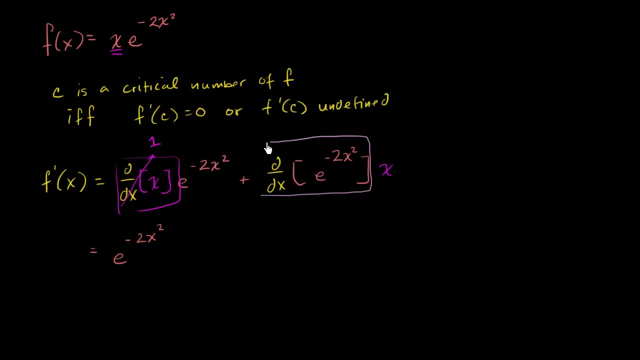 over here. I'll do this in this pink color. So this part right over here that is going to be equal to, or just apply the chain rule derivative of e to the negative 2x squared. with respect to negative 2x squared. 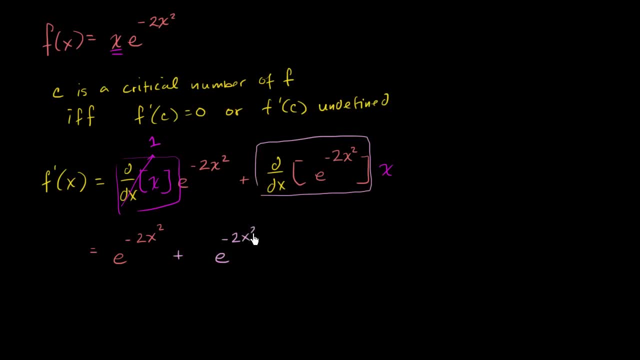 Well, that's just going to be e to the negative 2x squared, And we're going to multiply that times the derivative of negative 2x squared with respect to x, And so that's going to be what Negative 4x. 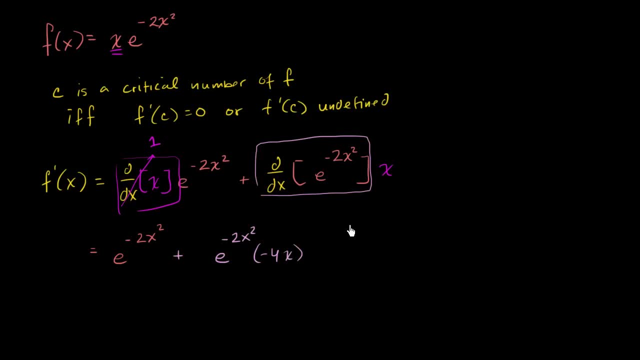 So times negative 4x, And of course we have this x over here, We have that x over there, And let's see, can we simplify it, Can we simplify it at all? Well, obviously, both of these terms have an e to the negative 2x squared. 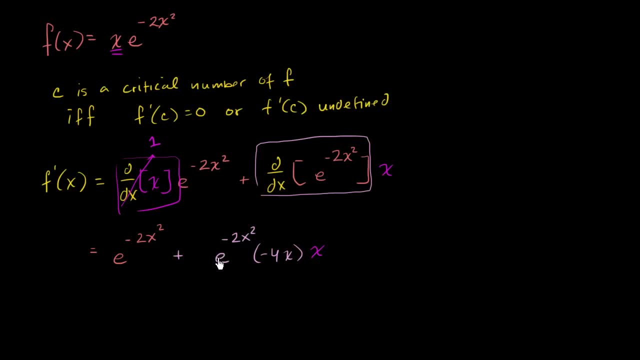 I'm going to try to figure out where this is either undefined or where this is equal to 0.. So let's think about this a little bit. So let's see if we factor in e to the negative 2x squared. I'll do that. in green we're going to have 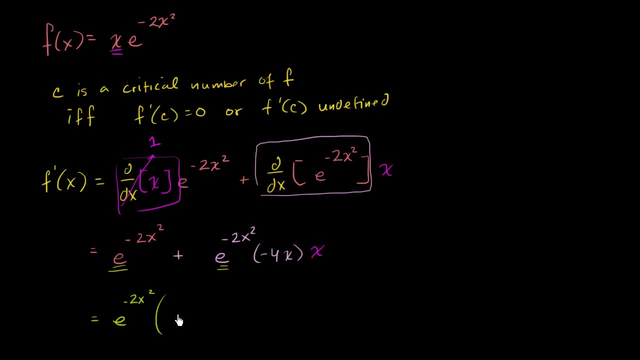 this is equal to e, to the negative 2x squared times. we have here 1 minus 4x squared. So this is the derivative of f. Now, where would this be undefined or equal to 0?? Well, let's see. 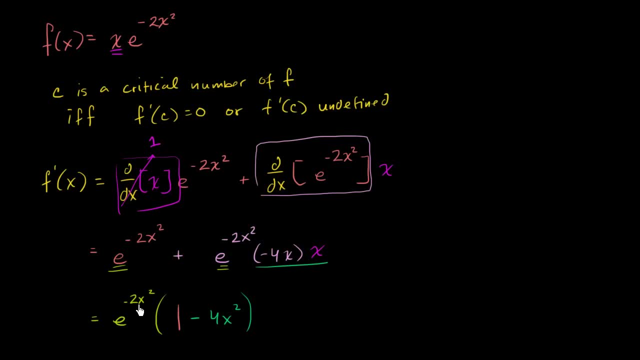 2x squared. this is going to be defined for any value of x. This part is going to be defined, And this part is also going to be defined for any value of x. So there's no point where this is undefined. But let's think about when this is going to be equal to 0.. 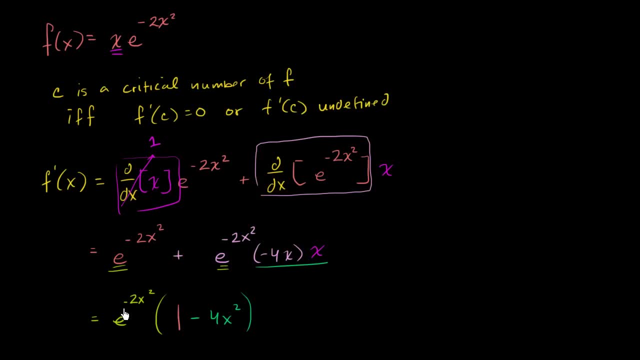 So you have this product of these two expressions equaling 0.. e to the negative 2x squared, that'll never be equal to 0.. If you get this exponent to be a really- I guess you could say- very negative number, you will approach 0.. 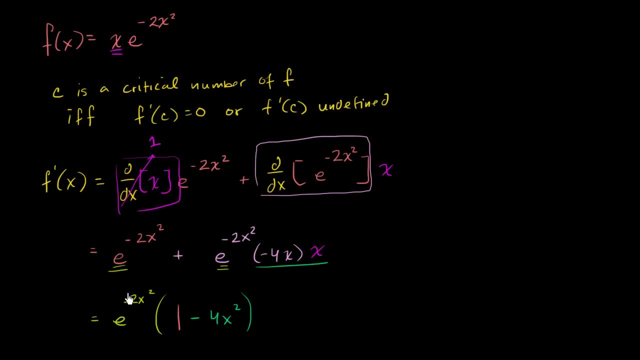 But you'll never get it to be. You'll never get it to be 0. So this part here can't be 0. But if the product of two things are 0, at least one of them has to be 0.. 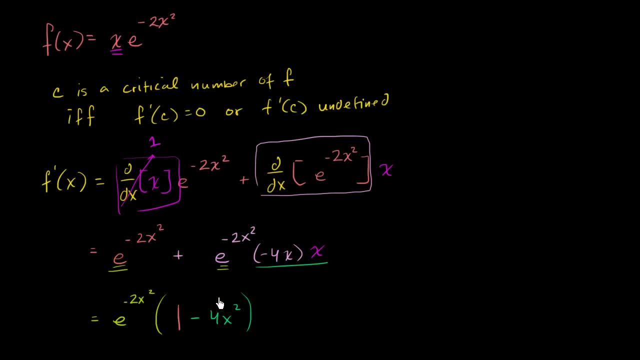 So the only way that we can get f prime of x to be equal to 0 is when 1 minus 4x squared is equal to 0.. So 1 minus 4x squared is equal to 0.. Let me rewrite that: 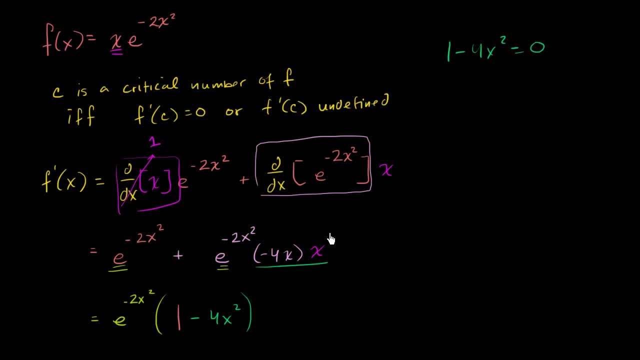 1 minus 4x squared is equal to 0.. When does that happen? And this one we can just solve. Add 4x squared to both sides. You get 1 is equal to 4x squared. Divide both sides by 4.. 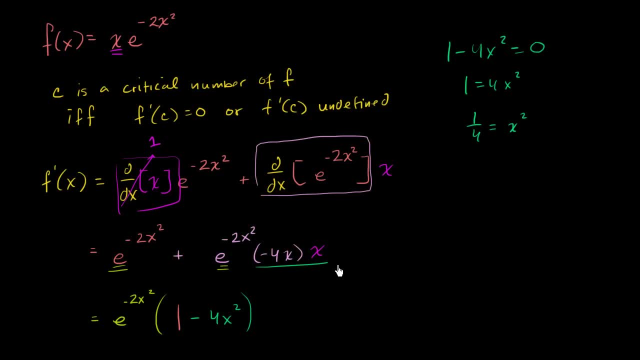 You get 1 fourth is equal to x squared. And then what x values? is this true at Well? we just take the plus or minus square root of both sides And you get: x is equal to plus or minus 1 half Negative. 1 half squared is 1 fourth. 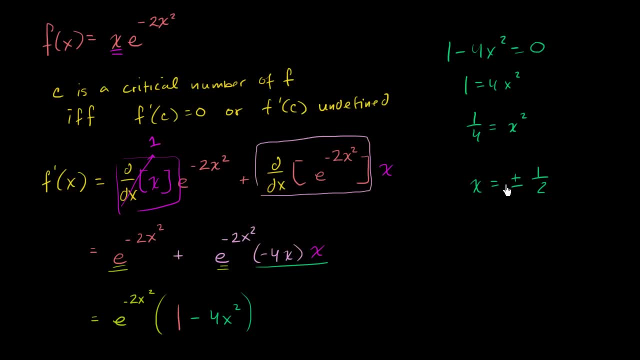 Positive 1 half squared is 1 fourth. So at x equals plus or minus 1 half. f prime, or the derivative, is equal to 0.. So let me write it this way: f prime of 1 half is equal to 0..